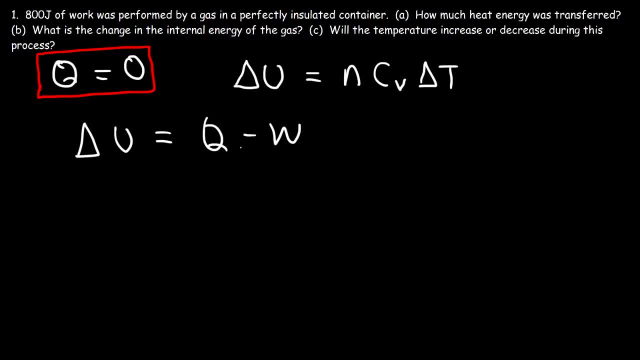 to Q minus W. Now, because Q is zero, delta U is going to be equal to zero minus W. So delta U is equal to negative W. Now we have W. It's 800 joules of work. Is W positive or negative? Notice that the work was performed by the gas, So W is positive. 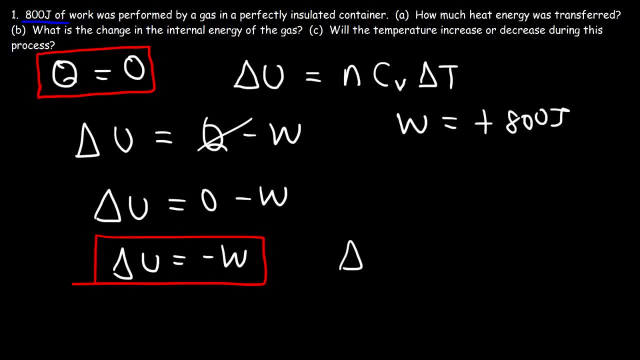 800 joules, which means that delta U is going to equal negative 800 joules. So this is the answer to part B. Part C: Will the temperature increase or decrease during this process? So delta U is negative. And keep in mind that delta U is equal to N, C, delta T. So if 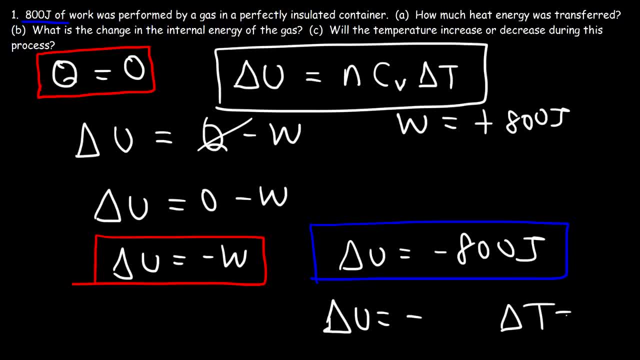 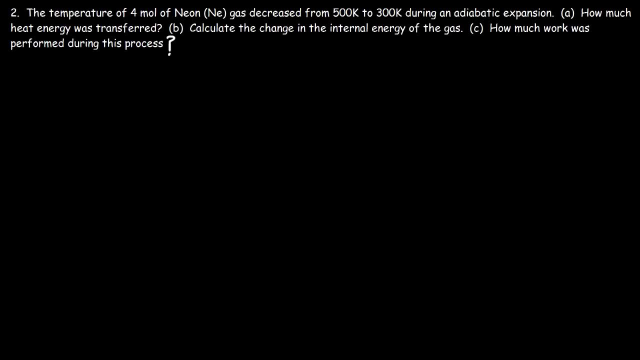 delta U is negative, that means that delta T has to be negative, which means the temperature has to decrease. Any time the internal energy of a gas decreases, the temperature will decrease as well, And so that's it for part C. Now let's move on to our next problem: The temperature. 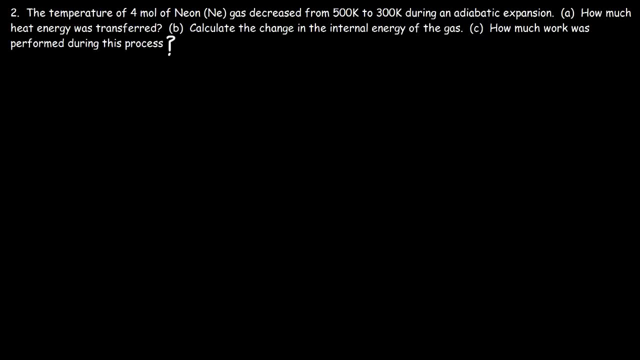 of 4 moles of neon gas decrease from 500 Kelvin to 300 Kelvin during an adiabatic expansion, How much heat energy was transferred? Well, for any adiabatic process, no heat energy will be transferred. so Q is equal to zero. So that's the first thing that you want to. 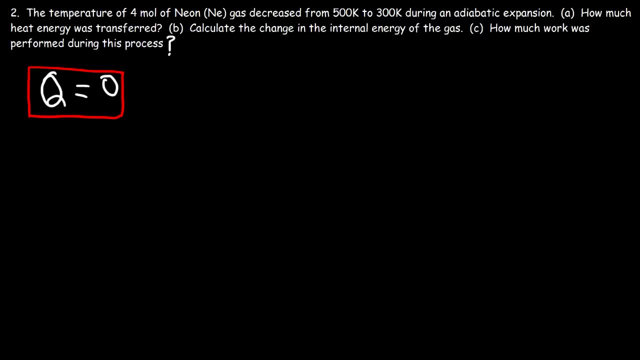 keep in mind for these types of problems. Now part B: calculate the change in the internal energy of the gas. So notice that we have a temperature change and we have the number of moles. So we could use this equation: delta U is equal to N. 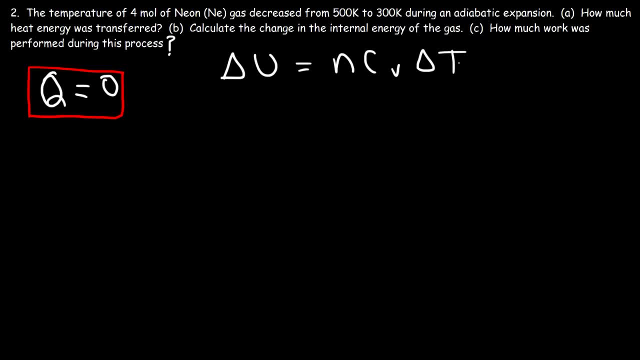 Cv, delta T. Now, the only thing that we're missing in this equation is the molar heat capacity at constant volume, so let's calculate that first. Now, what type of gas do we have? Neon? would you describe it as a monoatomic gas or a? 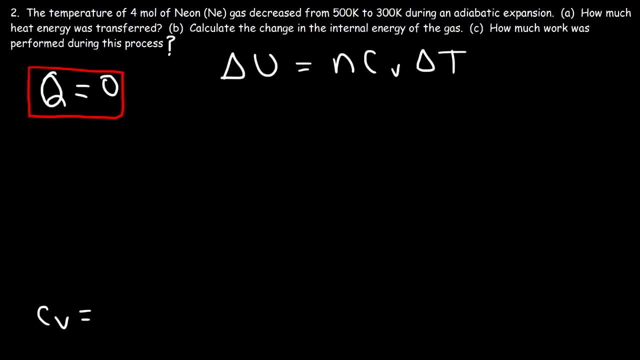 diatomic gas. Neon is a monoatomic gas. it has one atom per particle. So that's the number of moles that we have. Now part C: calculate the change in the. So it's equal to 3 over 2 times R. So that's 3 over 2 times 8.3145.. 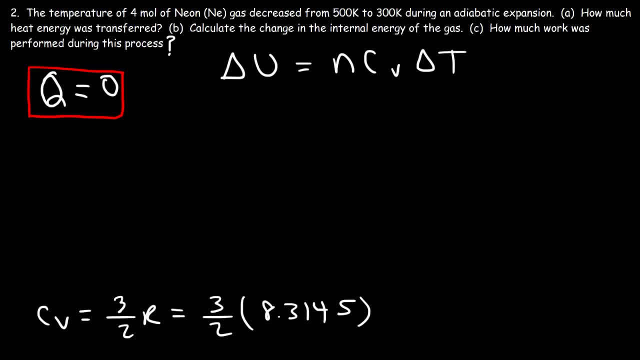 For diatomic gases it's 5 over 2R, So this is 12.47.. So delta U is going to equal 4 moles multiplied by 12.47 joules per mole per kelvin And the change in temperature. the final temperature is 300 kelvin. 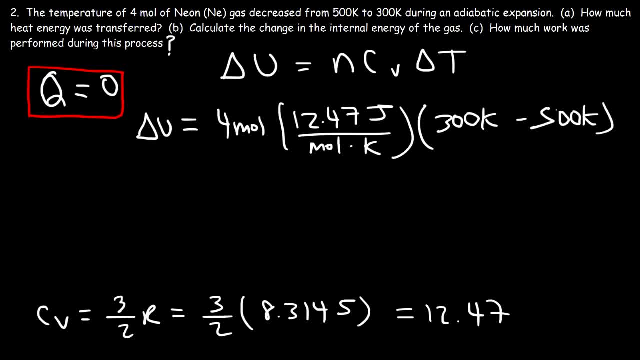 The initial temperature is 500 kelvin. So 300 minus 500 is negative 200.. So we need to take negative 200, multiply it by 12.47, and multiply that by 4.. So the change in the internal energy of the system is negative 9976.. 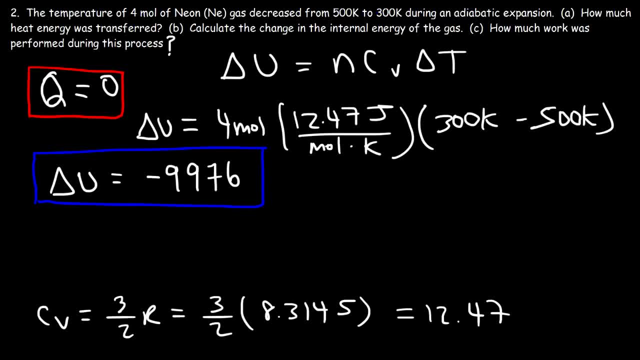 So, as we can see, because the internal energy decreases, the temperature decreases as well, from 500 to 300 kelvin. Now let's move on to part C. We know that delta U is equal to negative W, which means that W is negative delta U. 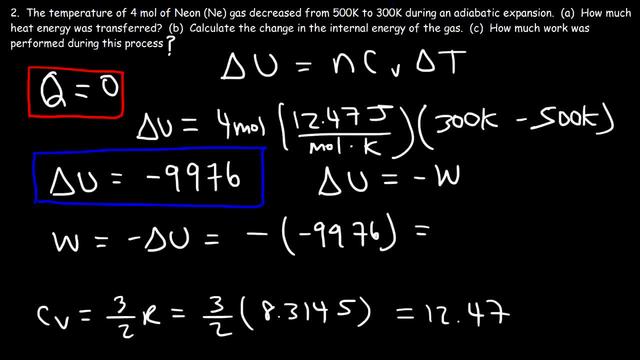 And delta U is negative 9976.. So the work performed during this process is positive: 9976 joules. The gas expands. the gas does work on the surroundings. the work is performed by the gas during an expansion. So W is positive for any expansion. 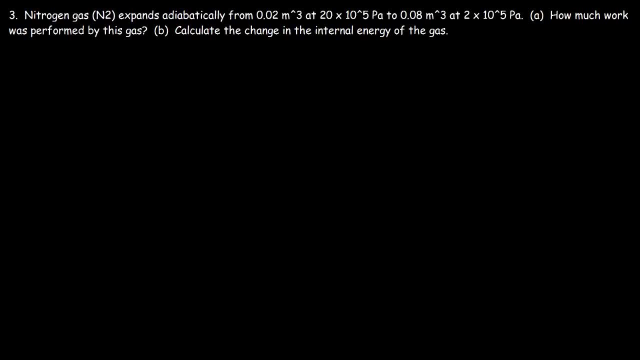 Number three: nitrogen gas expands adiabatically from 0.02 cubic meters at 20 times 10 to the 5 pascals to 0.08 cubic meters at 2 times 10 to the 5 pascals. 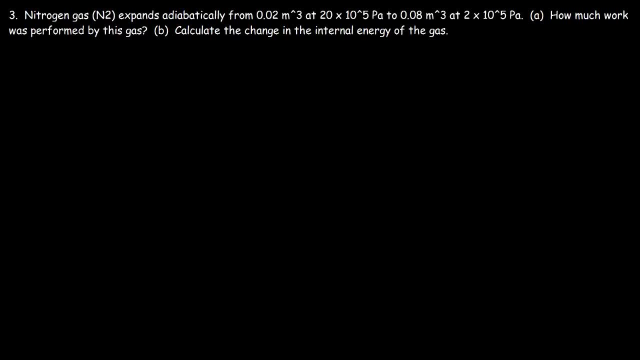 How much work was performed during this process? How much was performed by this gas? Another formula that you could use to calculate the work is negative Cv divided by R multiplied by the final pressure times, the final volume minus the initial pressure times, the initial volume. 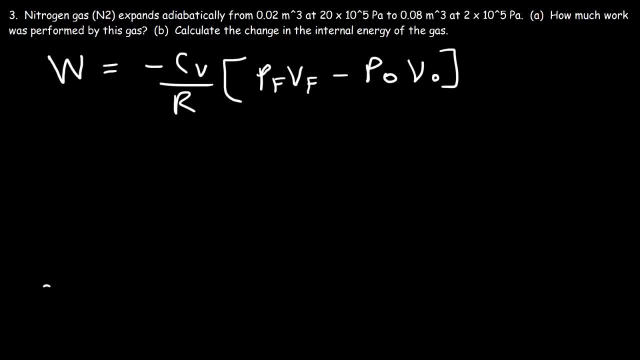 Now the only thing we're missing is Cv, And so this time we're dealing with a diatomic gas, because there's two atoms per particle, So it's 5 over 2 times R, And so that's going to be 5 over 2 times 8.3145.. 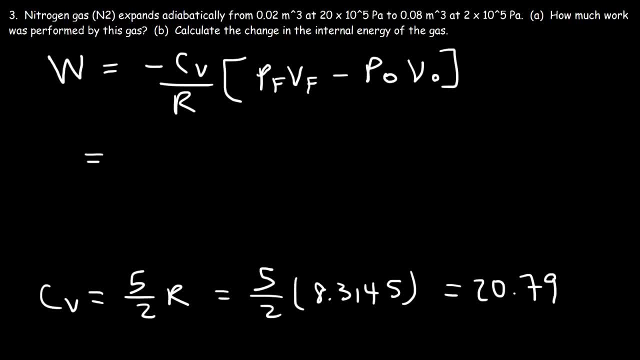 And so that's going to be 20.79.. So this is going to be negative 20.79 divided by R, which is 8.3145.. And then the final pressure, That's 2 over 2.75.. 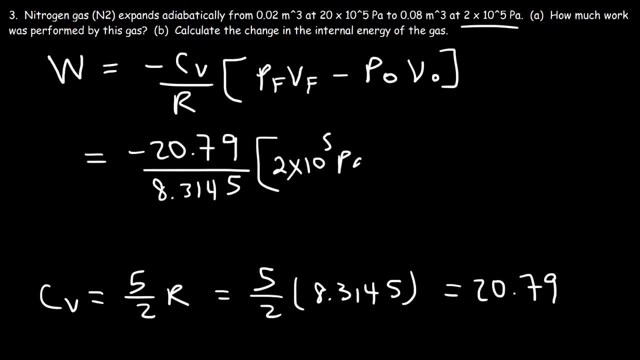 That's 2 times 10 to the 5 pascals, and we need to multiply that by the final volume, which is 0.08 cubic meters minus the initial pressure, of 20 times 10 to the 5 pascals times. 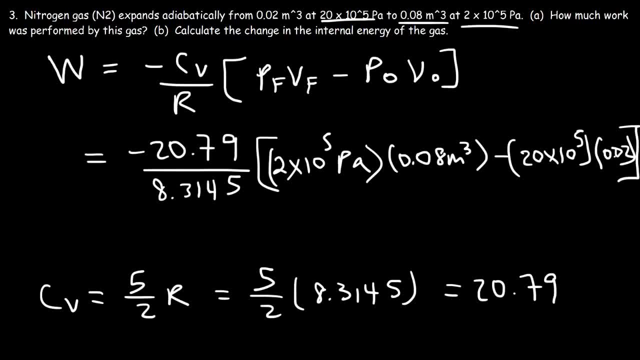 the initial volume of 0.02.. And I'm running out of space, So go ahead and plug that in. I'm going to do it one step at a time. So 2 times 10 to the 5 times 0.08.. 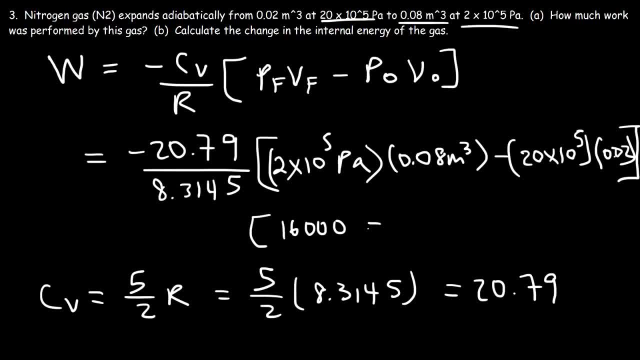 This is equal to 16,000.. And then 20 times 10 to the 5, multiplied by 0.02.. This is equal to 40,000.. And 20.79 divided by 8.3145.. That's equal to 2.5.. 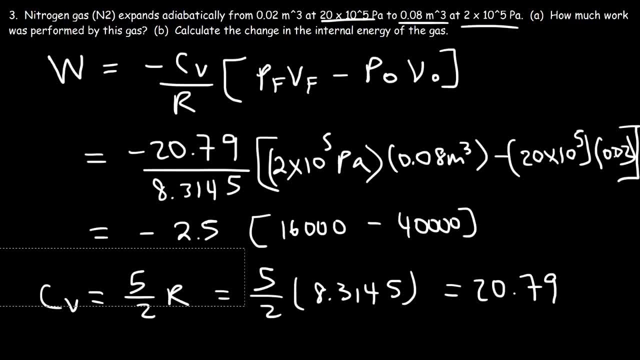 Okay, Okay, Okay, Alright, accounting That's good. Okay, let me turn this off. I want this back on. And then we run ourπεc prev lawsuit tests. So 16,000 minus 40,000.. So 16,000 minus 40,000 is negative 24,000 multiplied by negative 2.5.. 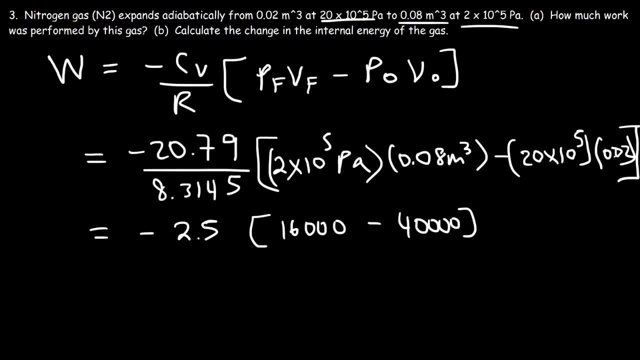 So that's equal to 60,000 joules and it's positive. And it makes sense because the gas is undergoing expansion. So work is positive for any expansion, expansion. So now we can move on to Part B, Calculate the change in the internal energy of the gas. 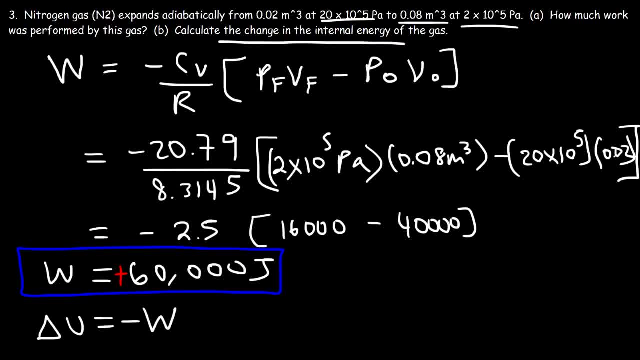 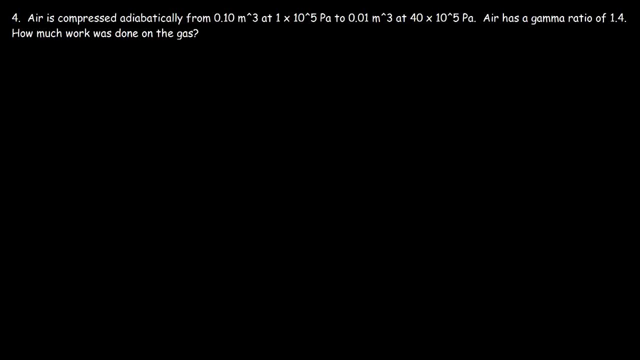 Delta U is equal to negative W for an adiabatic process, So it's going to equal negative 60,000 joules. And so that's the answer for Part B. Now let's move on to number four. Air is compressed adiabatically from 0.10 cubic meters at 1 times 10 to the 5 pascals. 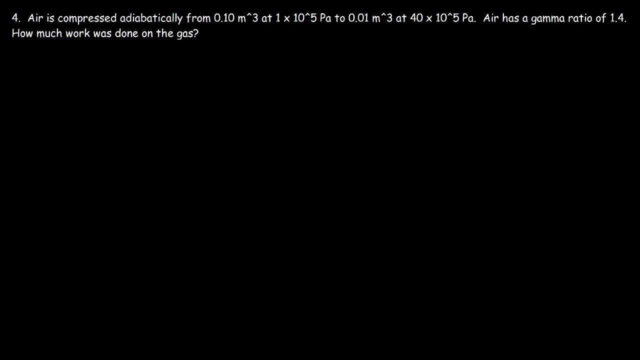 to 0.01 cubic meters, at 40 times 10 to the 5 pascals, Air has a gamma ratio of 1.4.. How much work was done on the gas? So the formula that we need for this problem is negative 1 divided by the gamma ratio minus. 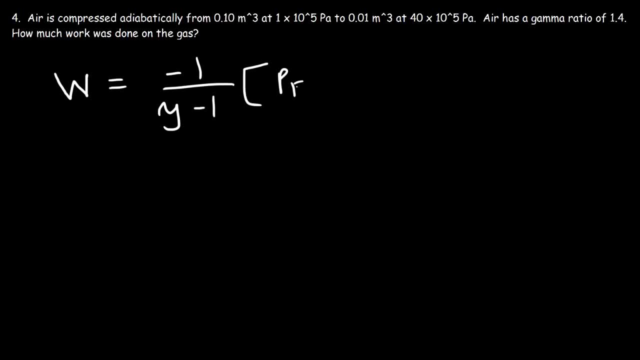 1, multiplied by the final pressure times the final volume minus the initial pressure. So the gamma ratio of air is 1.4.. The final pressure is 40 times 10 to the 5 pascals, The final volume is 0.01 cubic meters. 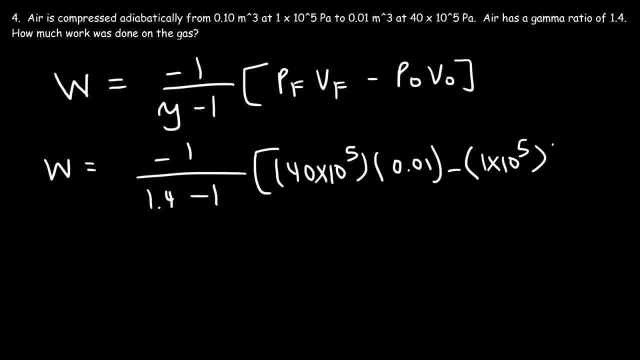 The initial pressure is 1 times 10 to the 5. And the initial volume is 0.10.. 1.4 minus 1 is 0.4.. And 40 times 10 to the 5, times 0.01, that's 40,000.. 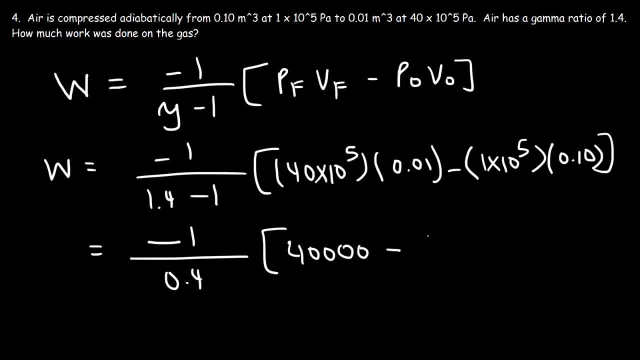 And 1 times 10 to the 5, multiplied by 0.1 is 10,000.. So 40,000 minus 10,000 is 30,000.. So this is going to be negative 30,000 divided by 0.4.. 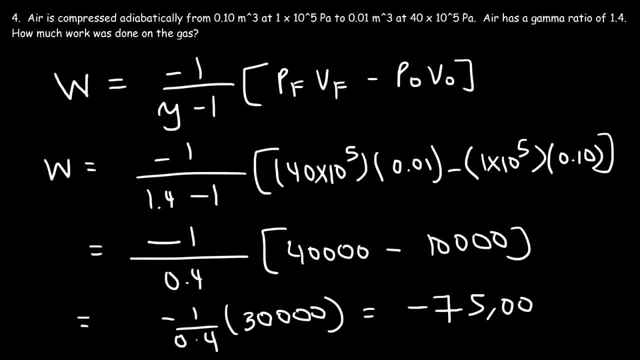 So the answer is negative 75,000 joules, Which makes sense, Because the gas is being compressed, the volume is decreasing, And so the work performed is going to be negative. Now, if we need to calculate the change in the internal energy of the system, that's: 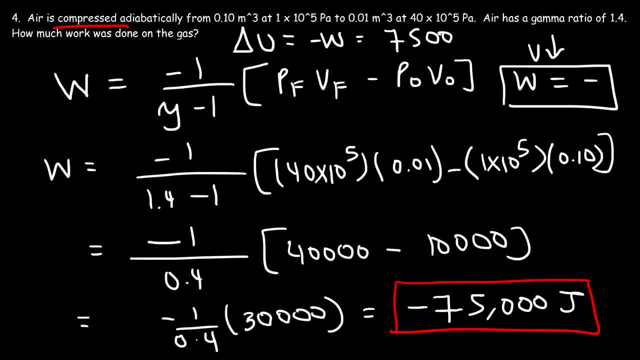 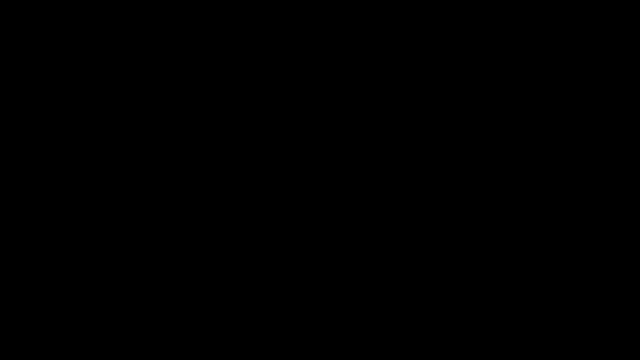 negative W And so that's going to be positive 75,000 joules, if we needed to get that answer. But that's it for this problem. Thank you so much. Thank you.